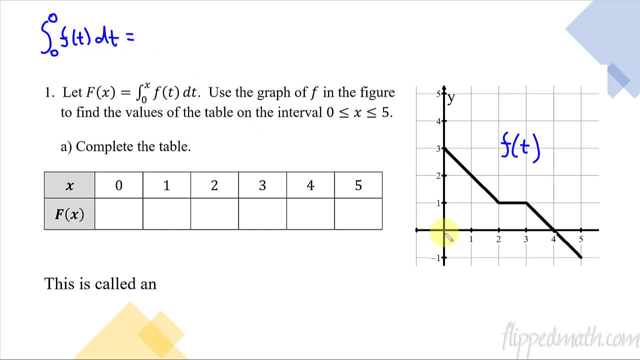 would equal if you go from zero to zero. the area from zero to zero is nothing. so that's easy: zero. And now if we do the next one, what that's saying is: if we go from zero to one of f. 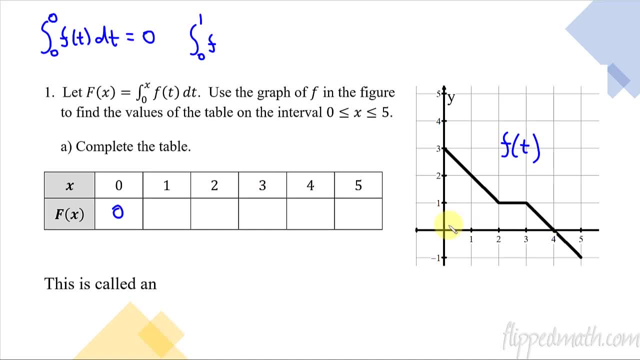 what is that? That's going from zero to one. so here we have this area here underneath that. so that's one square, two squares, two and a half squares. so this will be two point five, And now we're going to go from zero to. 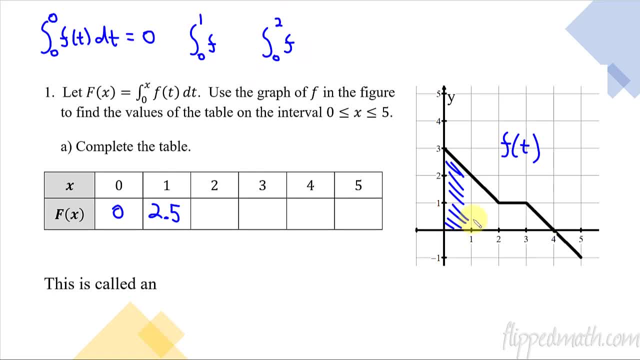 two of the function f. so now I'm going to go over one more and I get one block here, half a block there, so I'm adding one point five to the previous one. so I'm adding one point five to this, so that gets me up to four. So you can see. what we're doing is we are accumulating as. 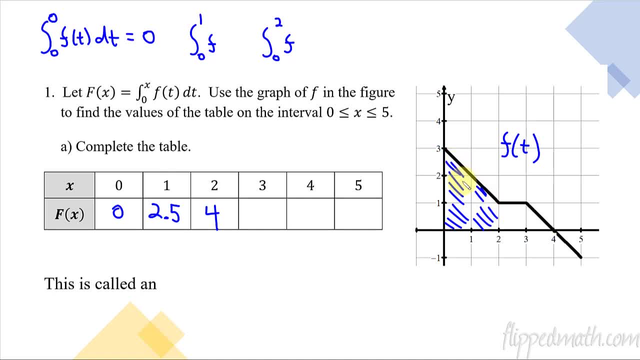 we go- Remember how we talked about accumulation, accumulation of change. That's what's happening. it's like we're accumulating this area as we add up. So if we go to three, now we're adding one more block, so now we're at five. and we're adding one more block, so now we're at five. 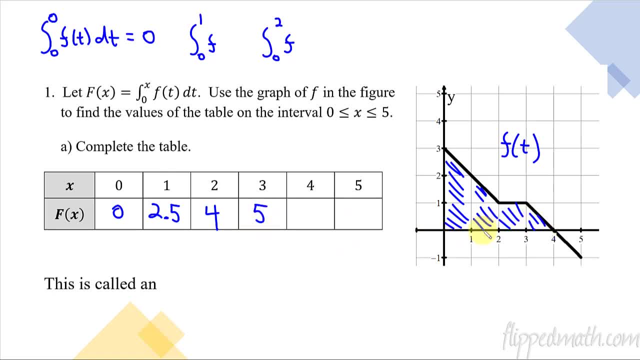 five, and then, if we go to four, we're adding half a block. so we're now at five point five, and then this last area. here it's now underneath the x-axis, so I'm going to subtract that and that brings us back to five. Okay, so here, and if I wanted to graph it, you could, let's see. 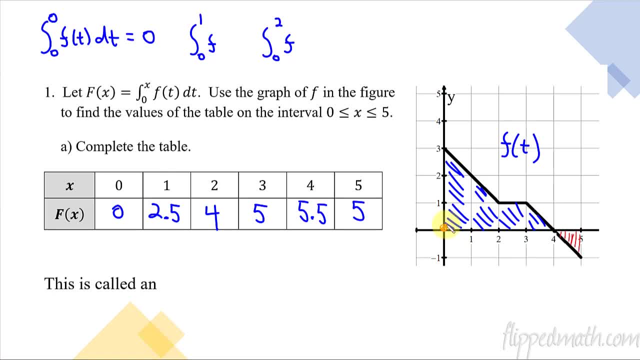 how orange shows up. so it would be zero, zero. I'd put a dot here. one and two, point five. one and two point five would be there. two and four would be here. three and five, three and fives up here. four and five point fives. off my grid a little bit. 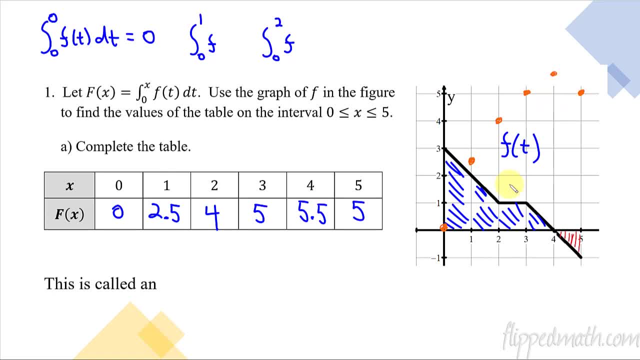 and then that would come back here. Okay, so that would be like a general idea of a shape of what this capital F- whoops that capital F- is doing. that's this little orange graph. So this is called an accumulation function. We accumulate as we go. 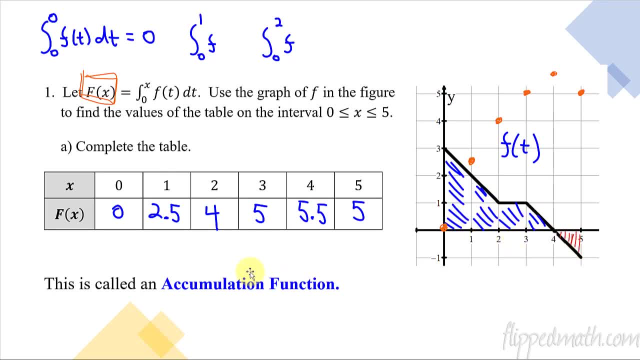 we might be getting bigger, we might be getting smaller, depending on the graphs above or below the x-axis, but that's what it is. When you have an integral, that represents a function, it's called an accumulation function. Now that leads us to the next important part of our lesson, which is: 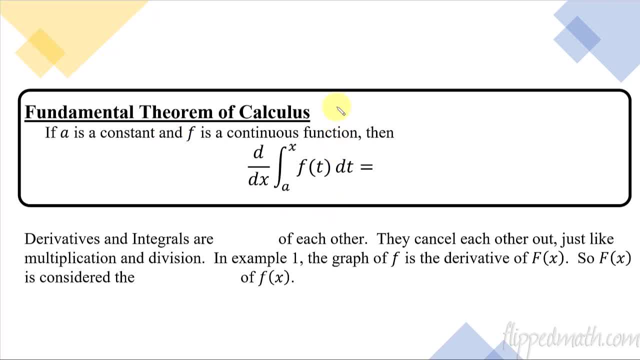 the fundamental theorem of calculus. Now I want to put in parentheses part two. And the reason I'm saying part two is because most textbooks and probably a lot of calculus teachers I've talked to actually teach this second. The reason I'm teaching it first is only because College Board 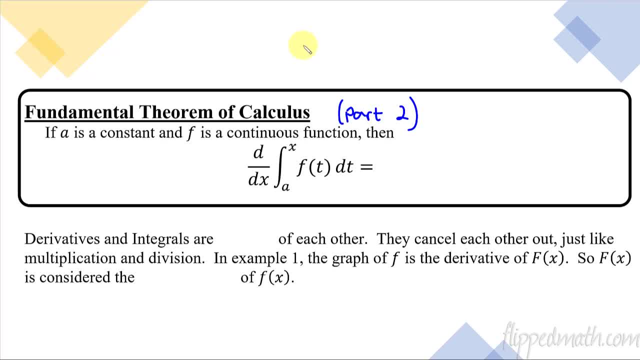 that I have seen- and I've checked with a lot of other things, calculus stuff- is that they teach this one second. It's okay if we learn it first, doesn't matter. I'm just referring to it as part two because you might see it in a lot of other places as part two. So later on in unit six, 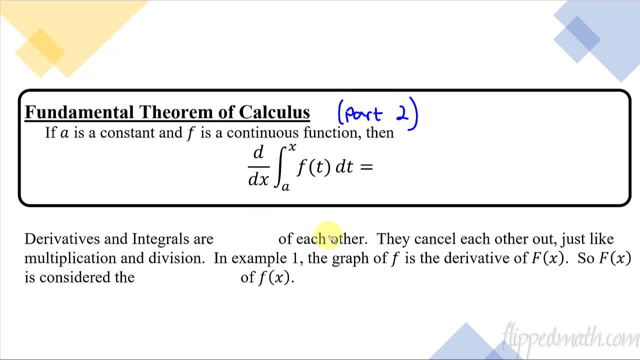 we'll do the part one of the fundamental theorem of calculus and they are tied together. So what this is is when you take the derivative of an integral and you're going from a to an unknown variable. when you take the derivative of that, what you get- this is crazy- is little f of x. 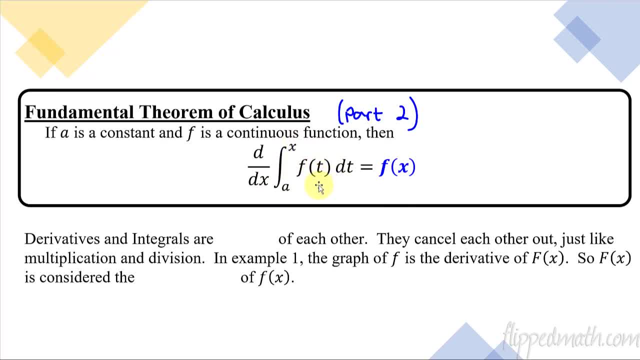 So if you have an integral and you take its derivative, you get what's inside here. In other words, derivatives and integrals cancel each other out. They're inverses of each other. They're inverses just in this way that multiplication and division are inverses of each. 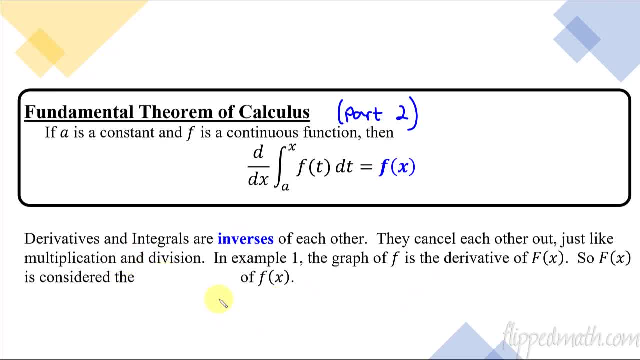 other. Like if you were solving an equation and you were multiplying, you'd have to divide to cancel it. That's what derivatives and integrals do? They cancel each other. So, derivative integral: you get what was inside. here It's called the integrand That's what this is. But so you 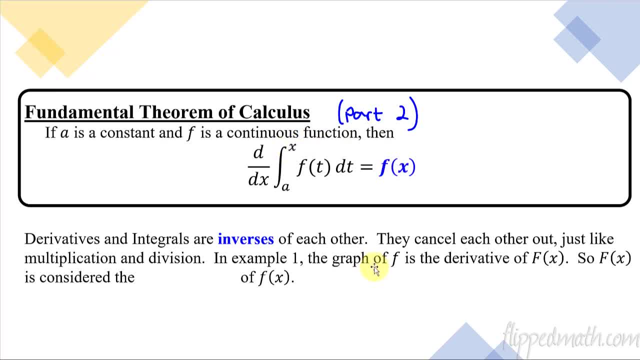 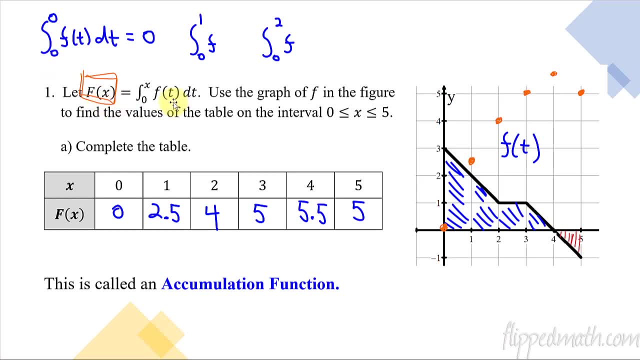 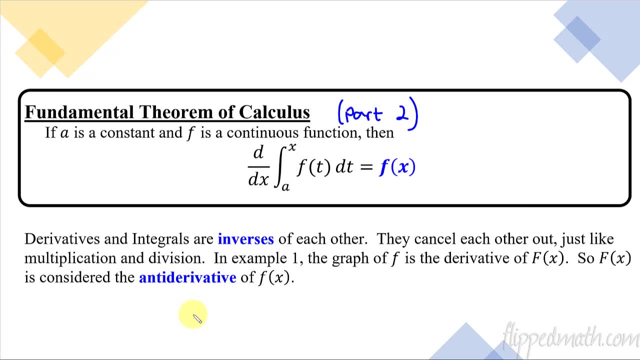 that just becomes this with the x plus. So let's go back to the graph. we were just looking at This capital F, this thing, and how it relates to little f. So if we have little f and we took the integral of it, what you get is the antiderivative. 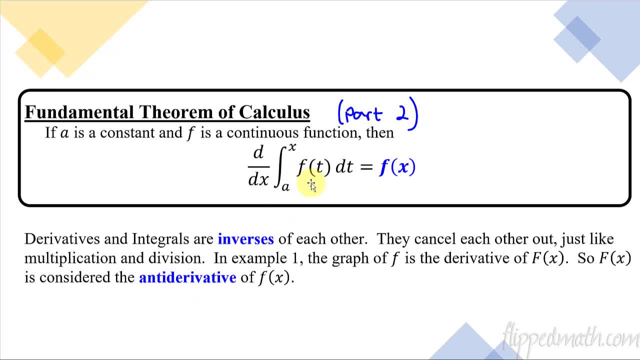 of little f. So the integral of something is the antiderivative. So the derivative of the integral gives you the little f, which means if you're doing the integral of this, you'd get the capital F, and that capital F is the antiderivative. Okay, Whoa, That was confusing, but trust me. 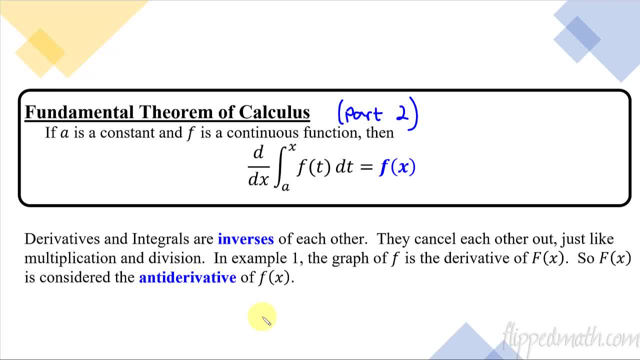 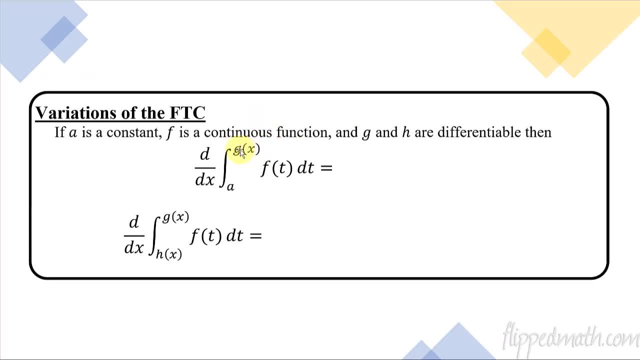 by the time we get done with Unit 6, you are going to crush this stuff. This really isn't that bad. So today's focus is going to be really simple. We're just going to practice taking the derivative of something that has an upper bound, that it is a variable, and that's all we got to worry about. 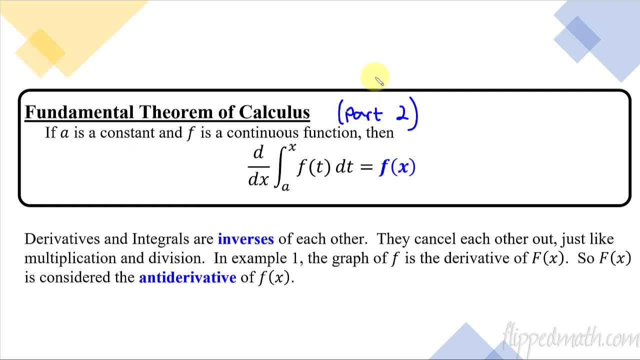 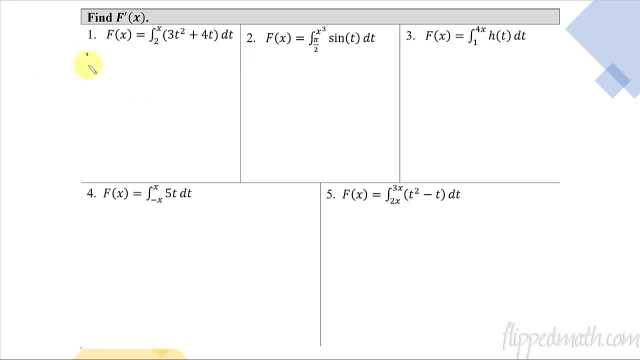 Now, before we do the variations, let's just practice what we did with this one. Let's just plug in this x for a really simple practice once. So notice, on this first example we are going to take, the derivative of this prime of x is going to equal. Now the bottom one, this two, it doesn't matter, It just had to be. 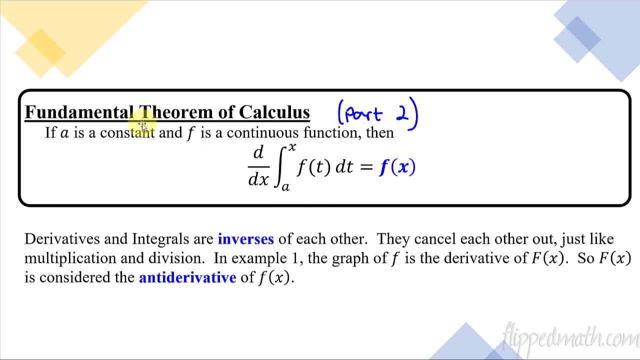 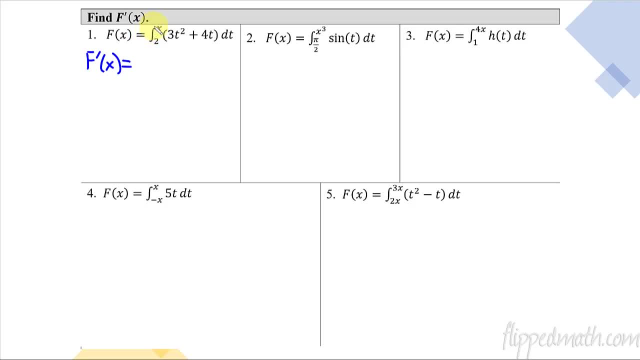 a constant. If you look back up here, the a is a constant and that's all it says. It doesn't say what number it is, just that it's a number. And as long as that happens, then all you do, the derivative of an integral cancels and that upper bound just gets plugged in. So it's just. 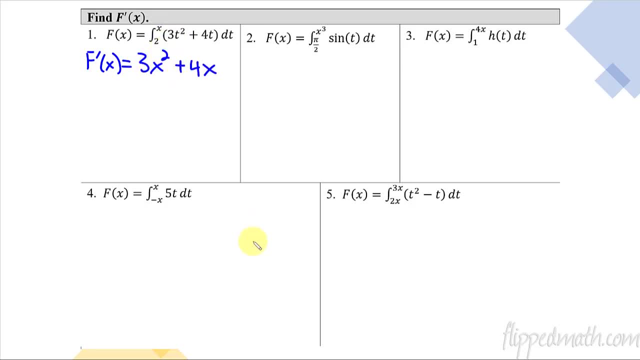 three x squared plus four x, and that's it. We're done That simple. Take the x, plug it in. Okay. so now let's do ones that are a little bit harder, which is the rest of these, but they're. 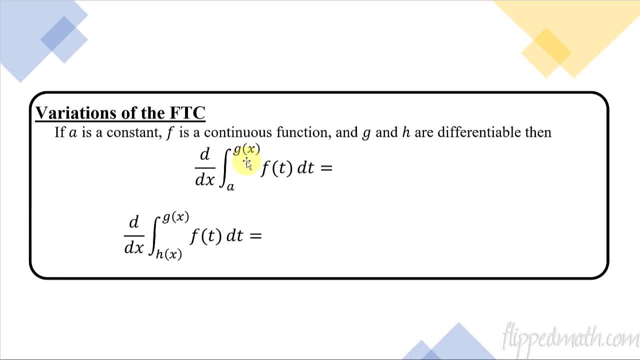 not that much harder. So this first one: sometimes it's not just an x, but it might be a whole expression up here, So I'm going to call it g of x. If you have that, you plug in the g of x still. 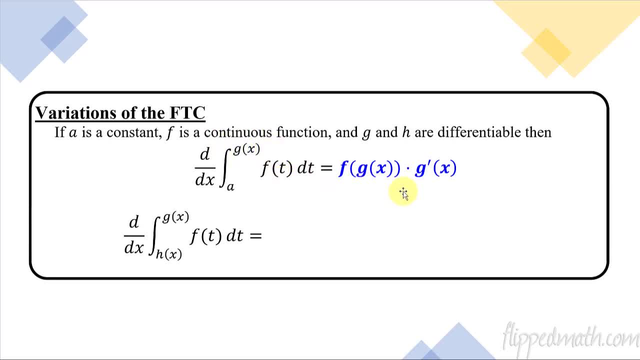 So you take this g of x, plug it into there where that t was, but then you have to apply the chain rule. Remember chain rule. the onion rule makes you cry. The chain rule is going to make us multiply by the derivative of what we just plugged in. So let's do a couple examples, just like that. 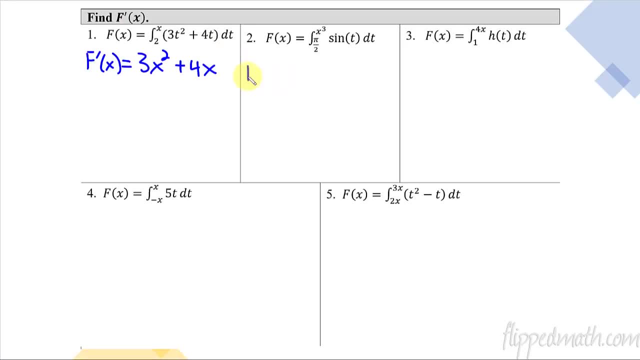 So this: we're going to take the derivative and there's not a lot of room here. The derivative of x is going to equal the derivative of f, prime of x, big F of x, is going to equal. take this x cubed. 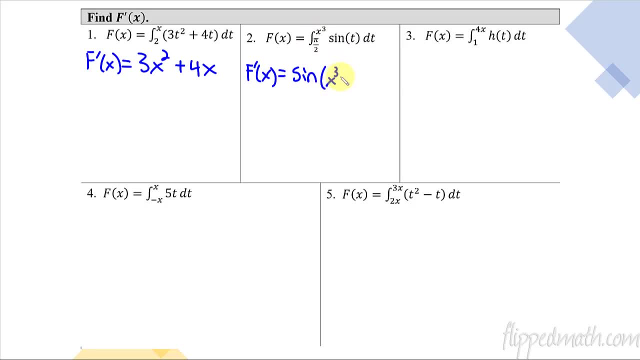 plug it in, So it's going to be sine of x cubed. And then you times that by the derivative of what you just plugged in, which is three x squared, And then, if we wanted, we could put that three x squared in front and make it sine of x cubed. Okay, so there is our derivative. 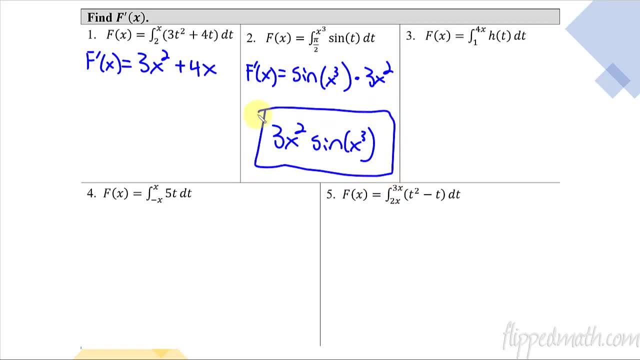 Of the big function f of x. Okay, this is the same idea. So there's there's a constant on bottom, something with variables on top. we are going to plug it in. So we get f. prime of x is equal. to plug it into the t, So it's just four x. And then you times that by the derivative of what. 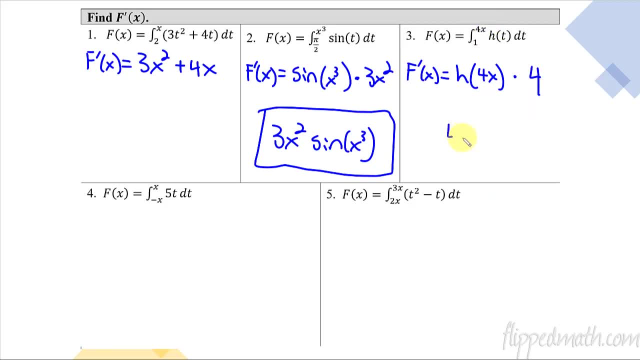 you plugged in. So that's the chain rule part. So times by four, And then we could change that to make the four like a coefficient. So it's four times h of x cubed, So that's the derivative of four x. We did in this case, we didn't need to know what h of t was, we just knew that it was a t. 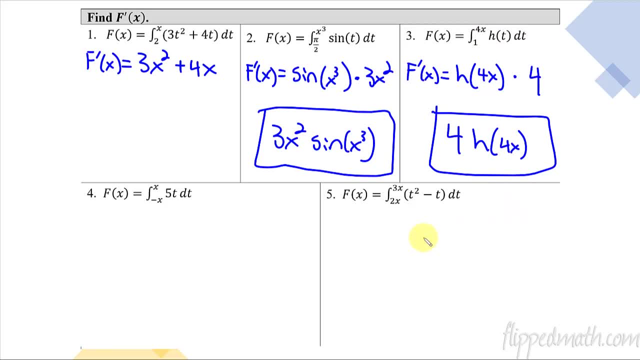 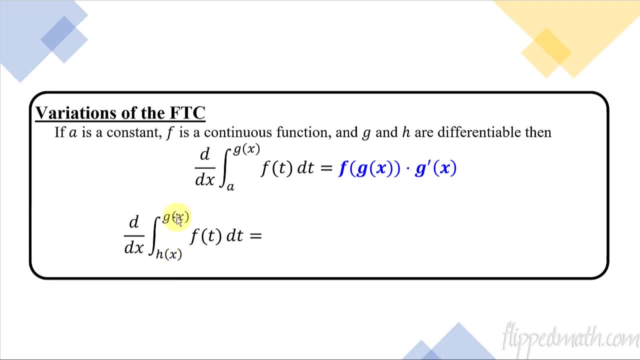 and then that gets plugged into the function there. Okay, so now let's go back and look at the other variation that we haven't done yet, which is when you have variables both on top and on bottom, So your upper limit and your bottom limit have variables in it- something. 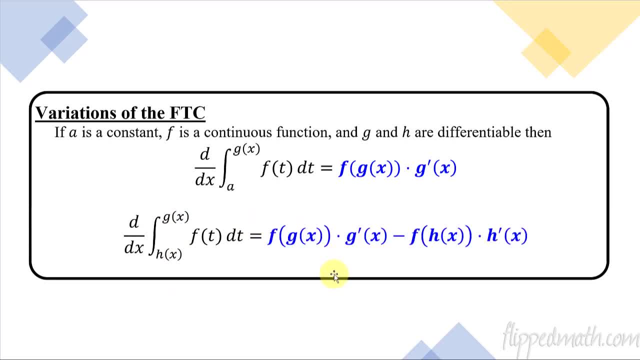 some expression involving x. So what happens in that case? this is what you get: this long crazy thing. Well, look at this: if we break it down, it's not that bad, Because this goes in like this. So what you're doing is you take the upper bound, you plug it into the function t. 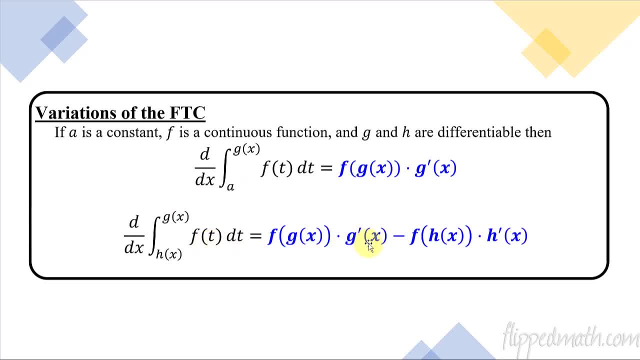 where f of t, plug it in and then do the chain rule times it by g prime. then you subtract the one that's on bottom. So we're going to subtract. then the h gets plugged in. So here's the h of x. 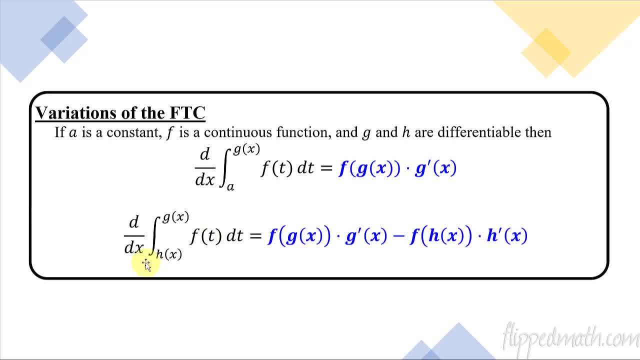 plugged into the f And you times that by the chain rule multiplied by the derivative of what you just plugged in. Okay, so it's almost like the one on top, except now you have to subtract the lower limit that gets plugged in. Okay, let's apply that. get that written down. 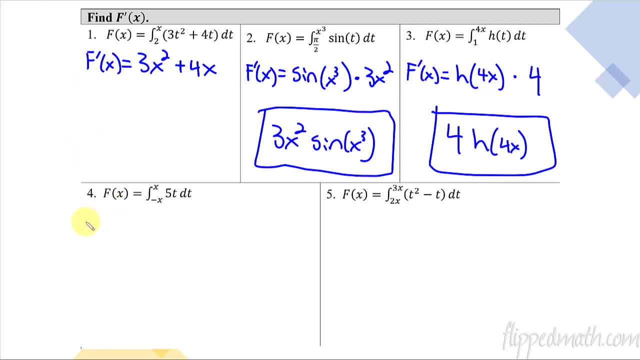 and then let's practice it with this. So I'm going to- I'm not going to write f prime just because I may not have enough room here- So just know, we're finding f prime. that's what we're doing on this next step. So take this x and plug it in, So we get five. 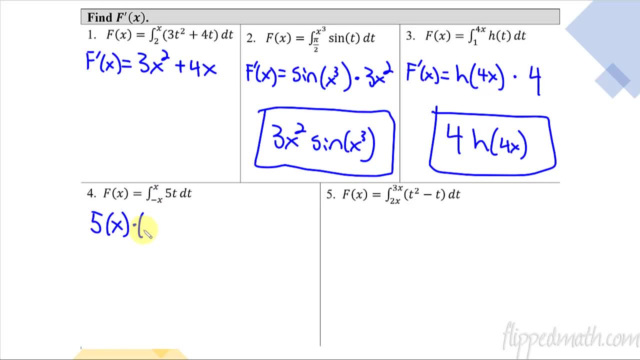 plug in the x and then you take the derivative of what you just plugged in, But in that case the derivative of x is just one. And then you subtract. And now we take this again, this function five t, and you plug in the lower limit, which is negative x times it by the. 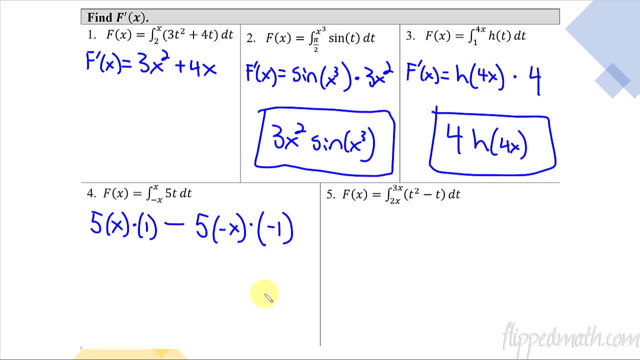 derivative of the lower limit, which is negative, 1, and now we simplify. this becomes 5x, a minus, and a minus is positive, but then another minus and so negative, negative, negative. that's going to give you a negative 5x, and that simplifies down to zero. okay, let's try this one. uh, this last one is going.